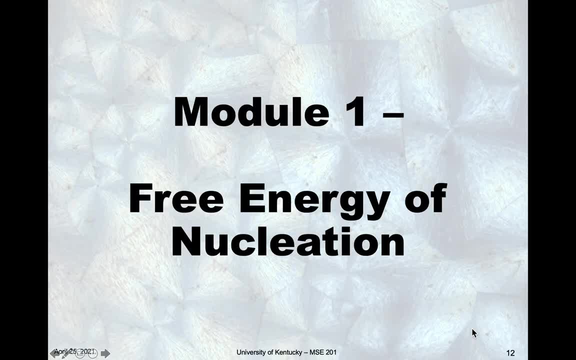 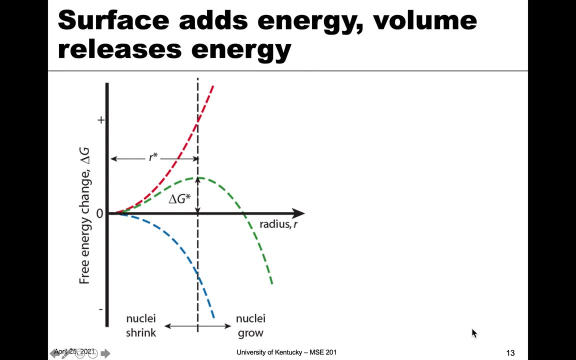 All right, in this module we're going to continue talking about nucleation and look at the free energy of nucleation. All right, so again we're talking about this concept of free energy, which you don't have to know everything about this. 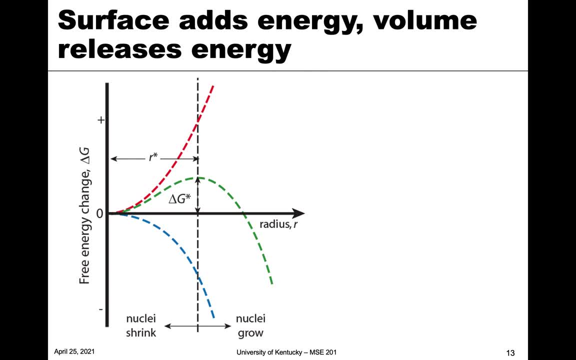 This is something that you learn more about in thermodynamics, But in a nutshell, it basically tells us what is favorable or what is not favorable. So basically, a negative value means that something is likely to occur. A positive it is not likely to occur. 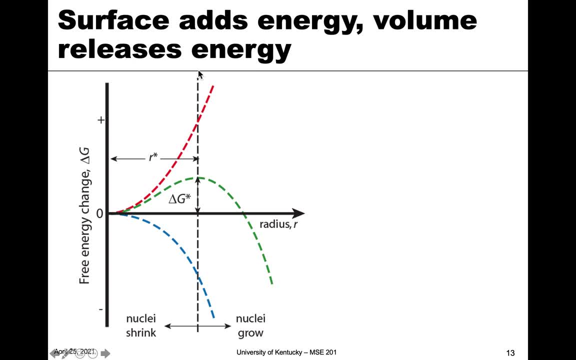 So that's the basics of it. So when we look at nucleation, we're actually going to look at two different terms that happen when we form a new phase. So the first one is this positive term In red here the red dashed- and this is related to the surface: free energy. 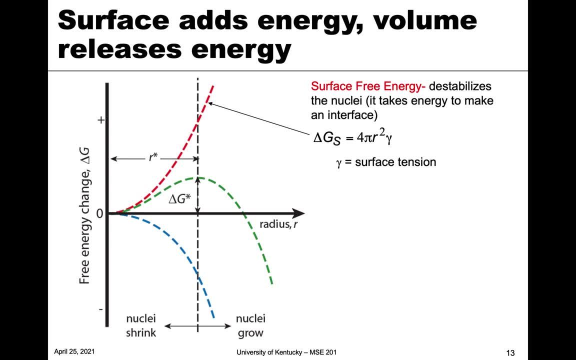 And what this is is it's the surface energy, that it's the surface area that's created between the solid and the liquid interface, And so this takes energy. This is not favorable to form a new boundary between solid and liquid, And so that's why this is positive. It kind of destate what we say is destabilizes. 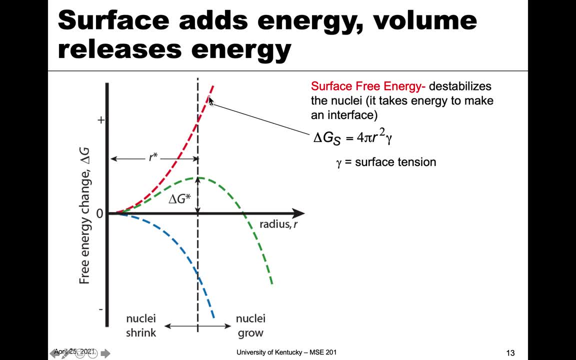 And so this will increase as the radius of the particle increases, right? Because the surface area will increase and therefore the energy will increase. So that's what the red curve is showing us, And so this can be related to the surface. free energy can be related to 4 pi. 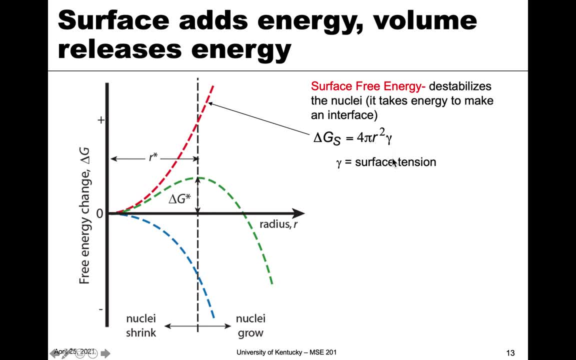 the radius squared of the particle multiplied by the surface, So that's what we call the surface tension between these interfaces. The other part that is stabilizing or favorable to the system is what we call the volume, or bulk, free energy, And so this is the free energy behind the formation of this new solid phase. 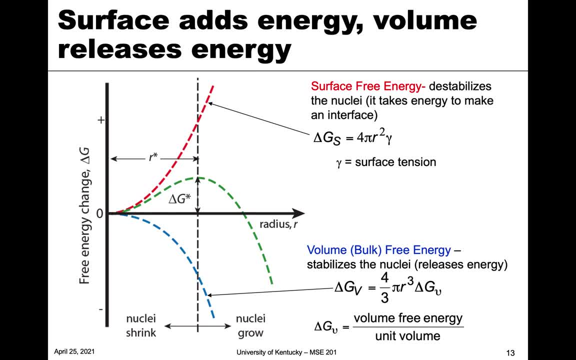 which, again, we know as favorable based on the fact that we're below the equilibrium temperature, And so this is related to the radius cubed because of volume right. So this is basically a volume term multiplied by the free energy per volume. 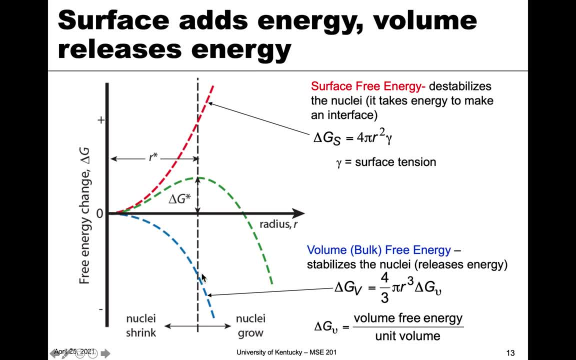 And so, in this case, the term decreases becomes more and more negative as the radius increases. But, as we know, this is r cubed and this is r squared. So this is going to do This is going to do this more rapidly than the surface term. 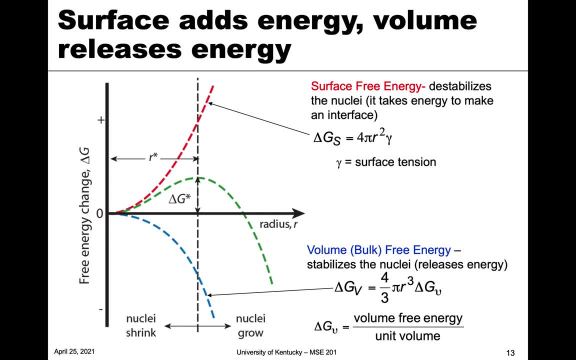 So when we look at the combination of both terms, which gives us the total free energy of the system, we're going to add those two terms together. right, And so when we do that, because this r cubed term decreases at a faster rate than the r squared term increases. 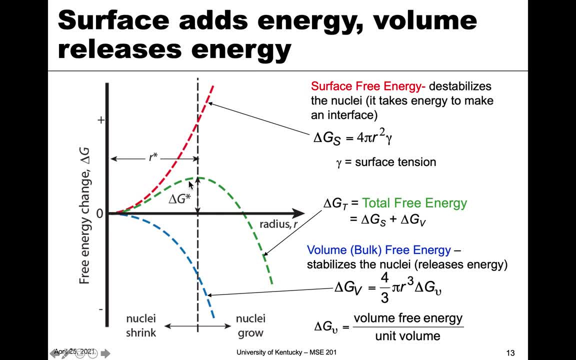 what we see is that initially, the total free energy increases becomes less and then the total free energy increases. And so when we do that- because this r cubed term decreases at a faster rate than the r squared term increases- what we see is that initially, the total free energy decreases. 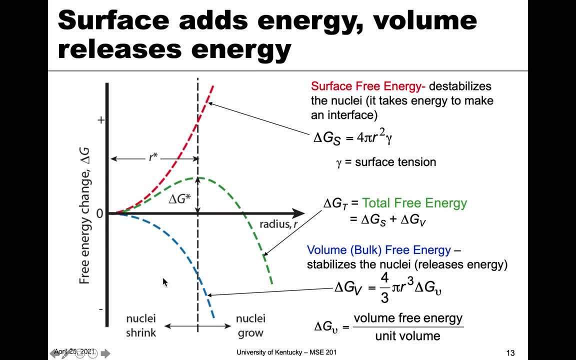 becomes less favorable. But at a certain point, when this volume term takes over, then we see it start to decrease and eventually goes negative, And so we see here that this is a maximum. So this is kind of a critical value in this scenario. 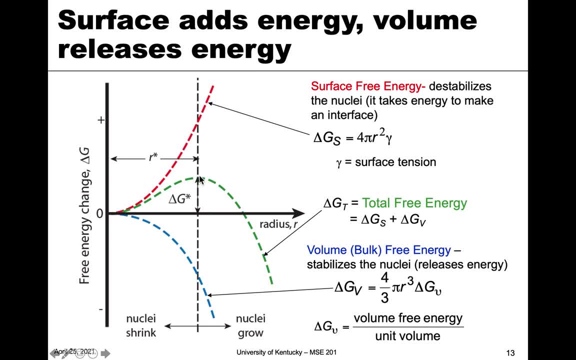 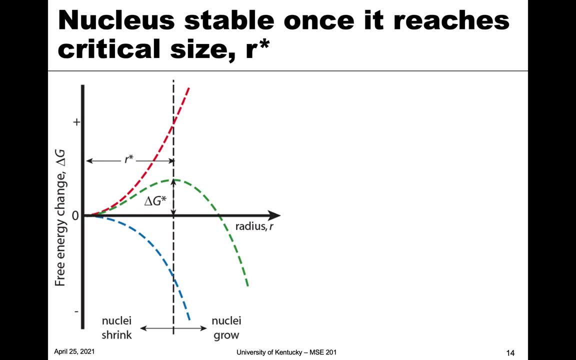 because this is the total amount of free energy that we would have to put in the system for this to occur. So, basically, what this is showing us is that this is a critical point. so we call this delta G star, because what happens is once the nuclei reaches the radius. here 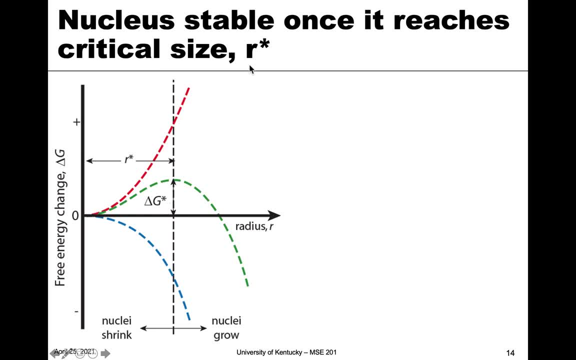 corresponding to this value. we call it r star. So this is r star, because that's the maximum amount that we have to put into the system. So for radii less than r star, the nuclei is just as likely to shrink as it is to grow. 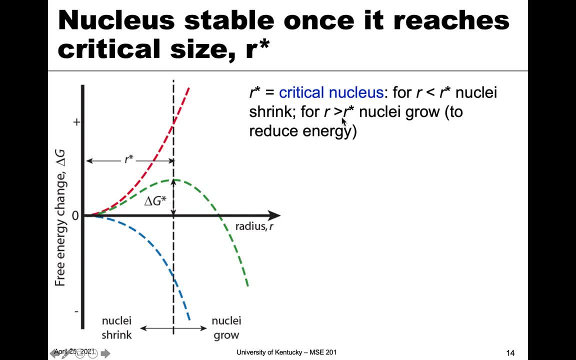 However, when the radius equals that r star or greater, then the nuclei is said to be stable and it will continue to grow to reduce the free energy of the system. So that's why we call this kind of the critical nucleus, because that's where it becomes stable. 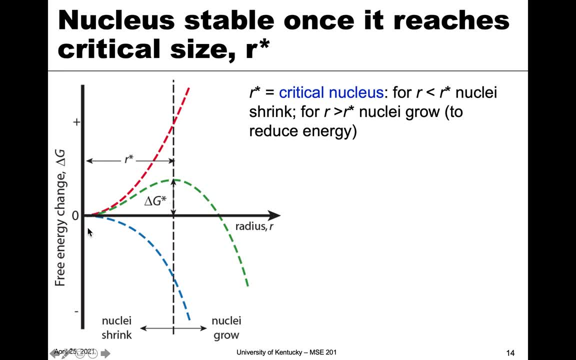 Below that, it's also likely to go back to liquid. So what we have to do is we basically have to supply delta G star's worth of energy to the nuclei before it becomes stable. So that's why we call it a critical value. 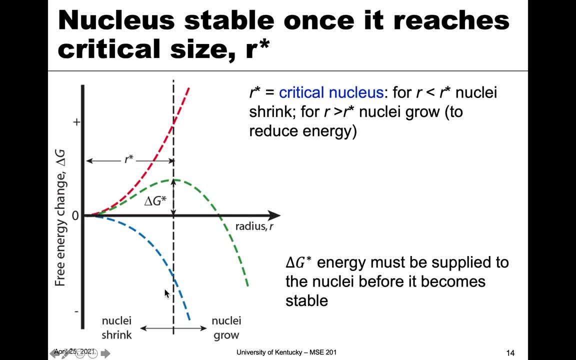 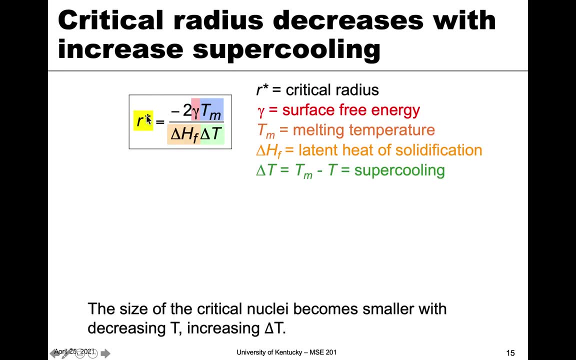 And so if we take the terms for volume and surface and add them together, we saw that we had that and we can actually solve for this maximum and solve for r star by looking for the maximum of this equation. And if we solve for that, 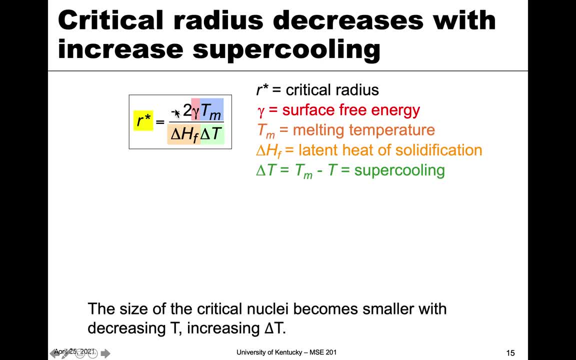 we see that the critical, the critical radius r star is equal to minus two times the surface tension or surface free energy multiplied by the melting temperature, divided by the latent heat of solidification, so the enthalpy multiplied by the super cooling, so delta T. 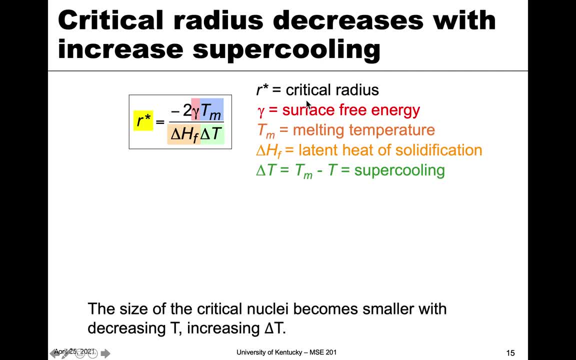 And so this allows us to calculate the r star for the system, And what we see is that it's going to be a function, an inverse function of the delta T, the super cooling term. A couple other notes to mention here. So enthalpy and surface energy are weakly dependent on this temperature. 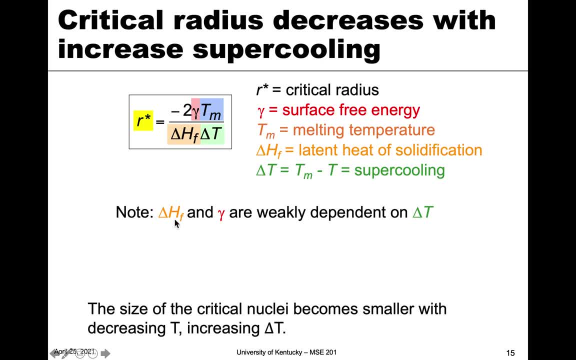 but not as much as the r star. So it's just a. couple of these can change with temperature, but for the most part they're only weakly dependent. So what we see is that r star will decrease as super cooling increases. 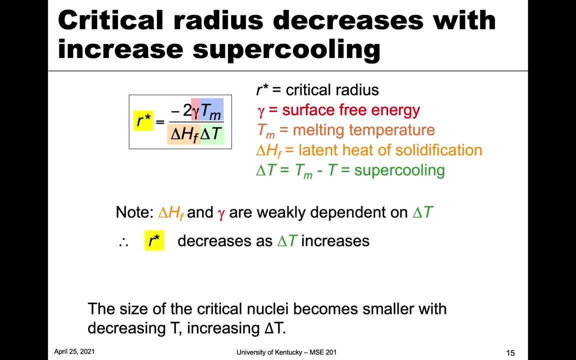 right. So the temperature decreases overall, So the size of the critical nuclei becomes smaller with decreasing temperature or increasing delta T. And so if you're wondering some, some approximate values here, what these values tend to be, So for typical degrees of super cooling, 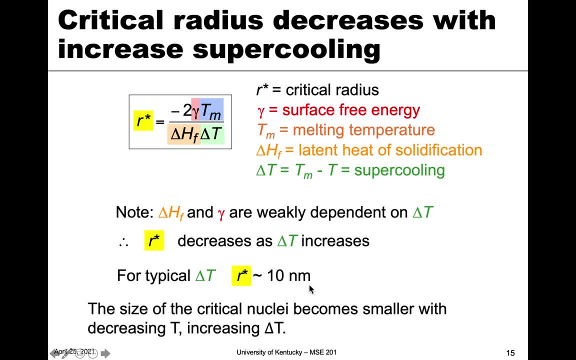 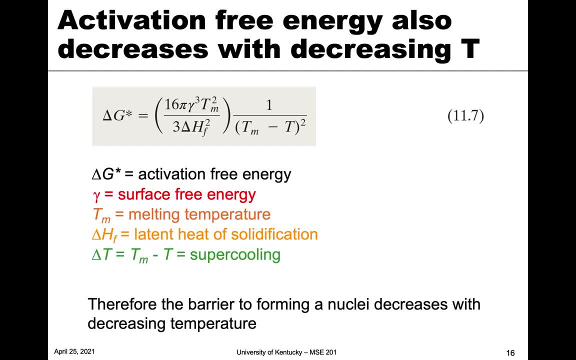 um, the critical radius is about 10 nanometers, right. So that's when it becomes critical. So about 10 nanometers, All right. So along with that we can calculate the delta G star, And that's when the